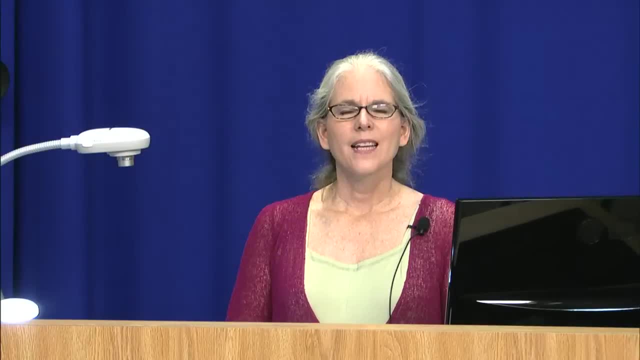 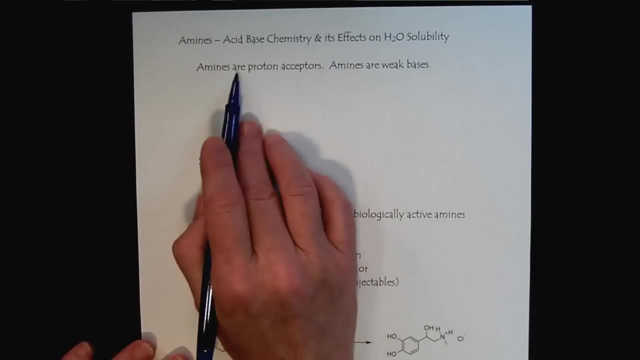 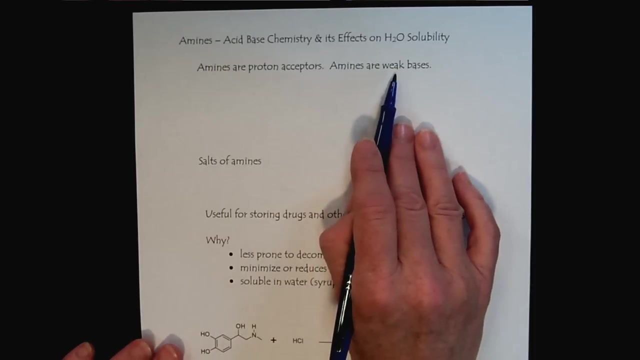 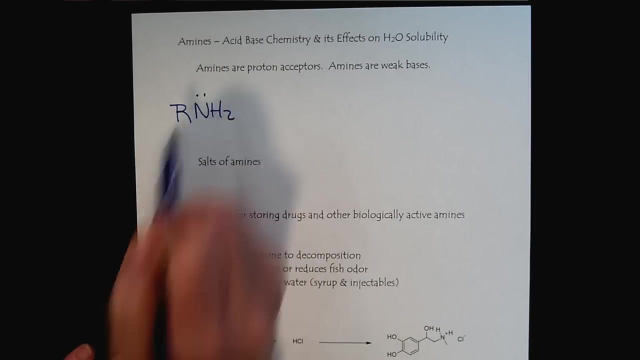 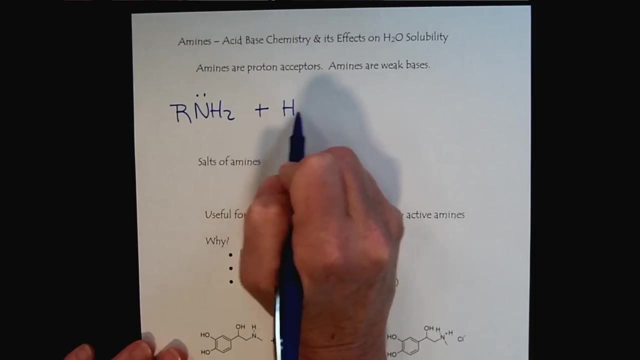 Welcome to a video tutorial that will introduce the acid-base chemistry of amines and especially how it's related to water solubility. Let's get started All righty now. amines are proton acceptors and so that's a base, and particularly they're weak bases. So we'll draw a generic structure for an amine and we'll just do a primary amine to keep things simple, and then we will react that with an acid such as hydrochloric acid, and because hydrochloric acid is a strong acid, we will show a complete 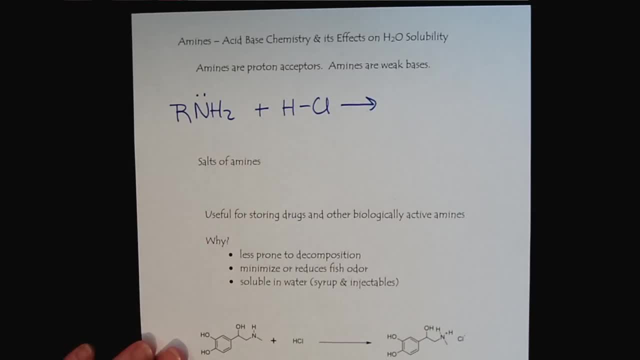 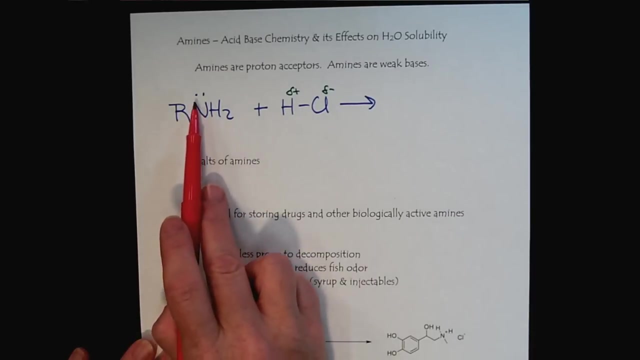 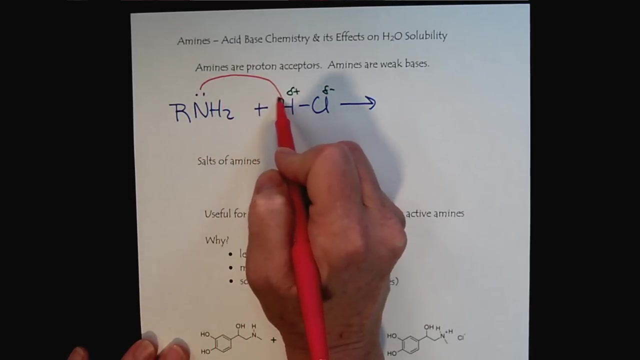 reaction arrow. So if we think about our understanding of electronegativity and polarity, we know that there's a partial positive and a partial negative here and we have some lone pair electrons. So electrostatically, even though this is neutral, the negative charge of those electrons is attracted to the positive charge of the hydrogen ion and hydrogen can only form one bond. 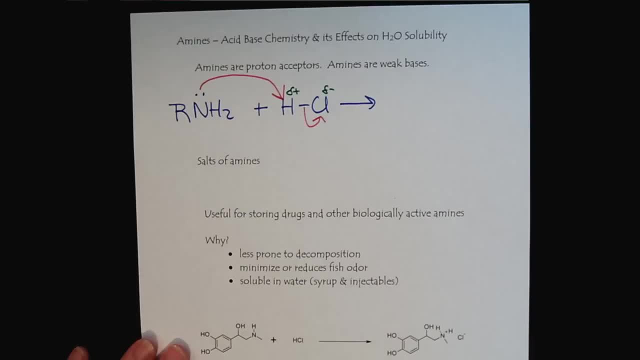 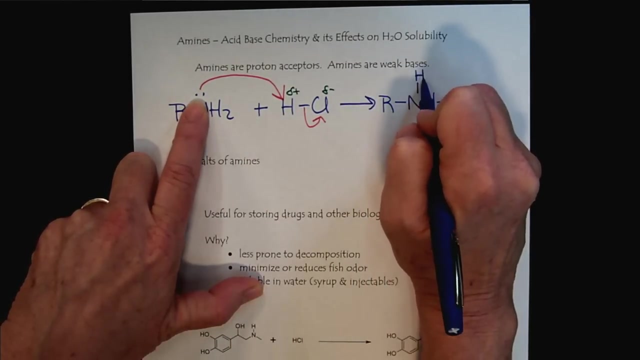 And chlorine is electronegative, so we get this a reaction occurring. So you're not responsible for this reaction, but I think it helps with the understanding why things are going on. So now I'll draw the product, and so I'm going to leave this part the same, and then this lone pair is what creates the bond to the hydrogen atom. 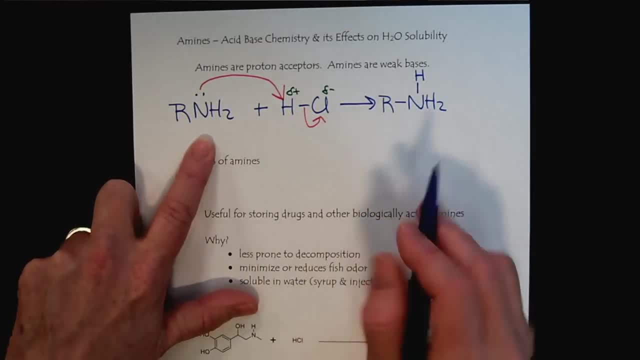 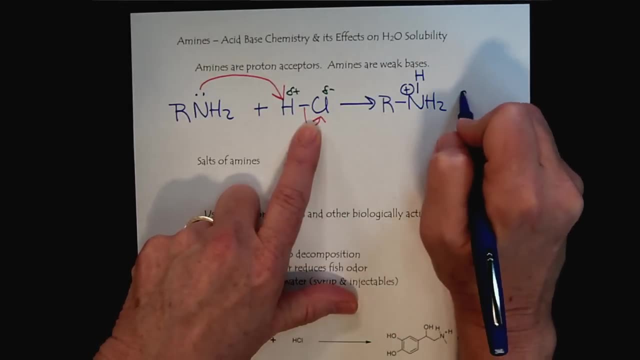 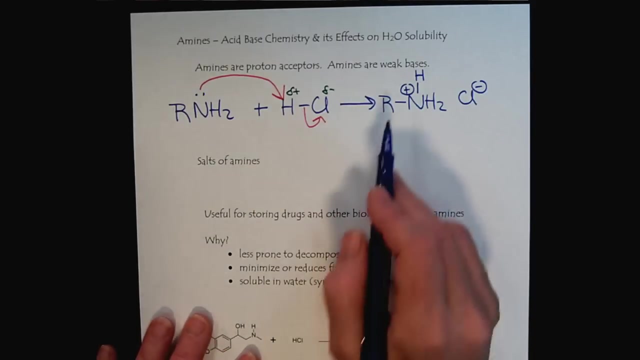 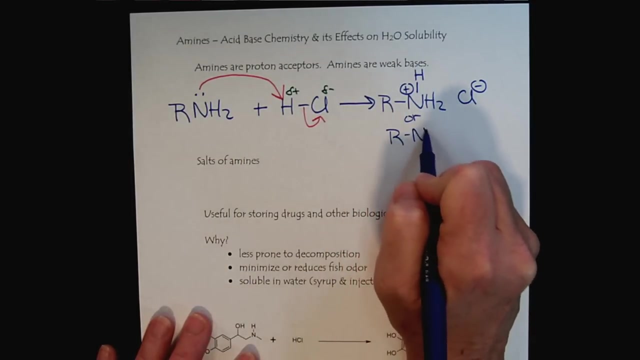 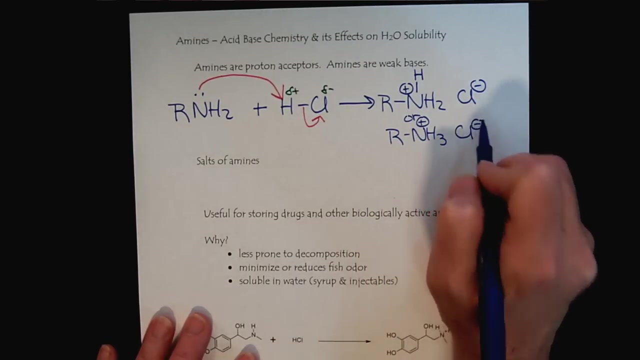 Now our nitrogen is no longer in its neutral bond, It's in its bonding pattern, so it will have a positive charge and the two electrons here are now alone or completely with the chloride. There's another way to draw this, so I did this to help you see what's going on in the reaction. and we could simplify this and put all of the hydrogens together with the positive charge, and then there's the chloride. 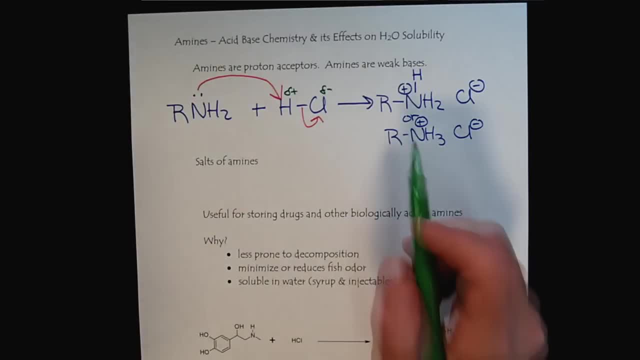 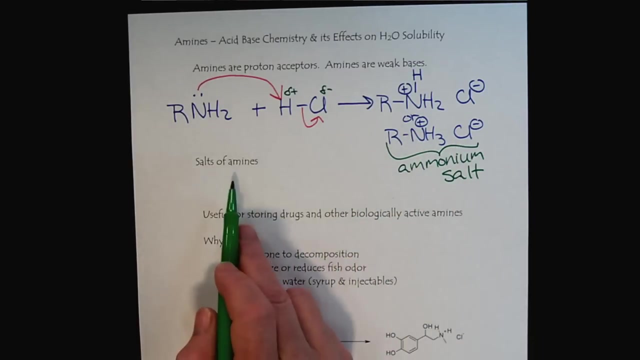 So this is very important. here. We describe this as an ammonium salt, So it's a more complicated ionic compound because we can have a large complex R group, but it's still fundamentally a cation and an anion. And so these salts of amine, these are very important because 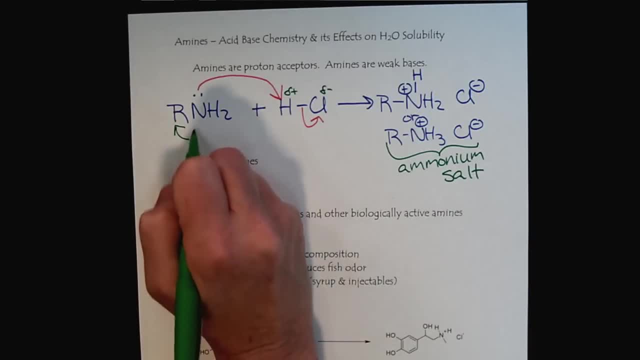 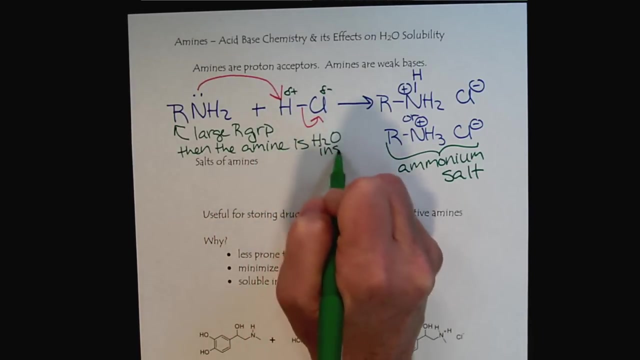 the R groups can be very large, right? So if we have a large R group, then the amine will be water-insoluble, No water solubility or very low. So just like we saw in the carboxylic acid tutorial, 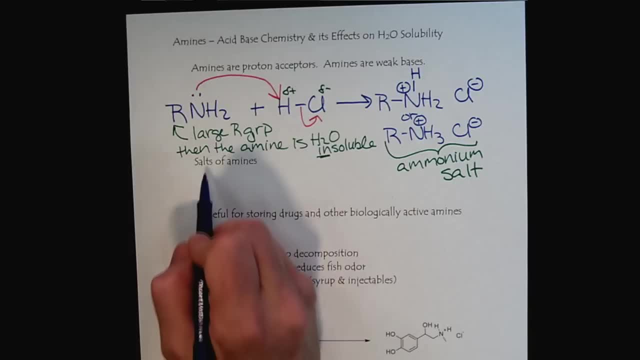 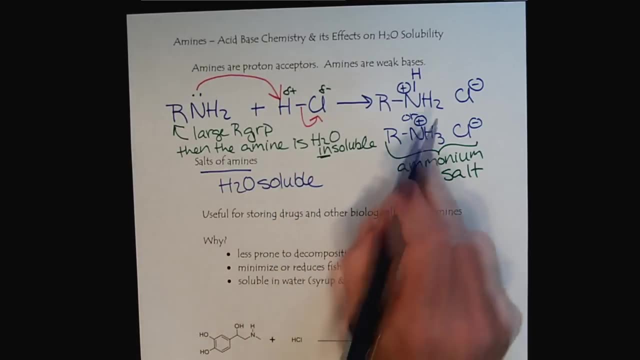 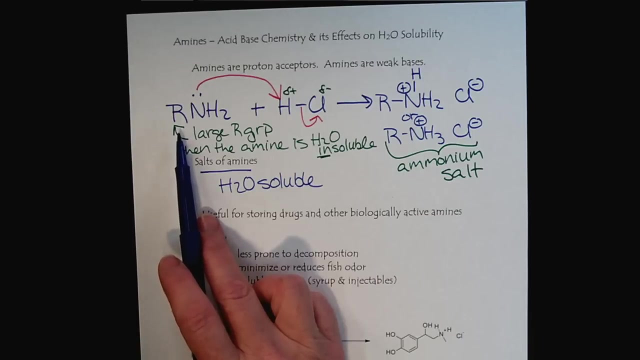 if you have, if you've watched that one already. the salts of amine are water-soluble. Right, It's the power of charge. Having that full positive charge can overcome the hydrophobic qualities of the large R group. So the salts of amine are water-soluble. 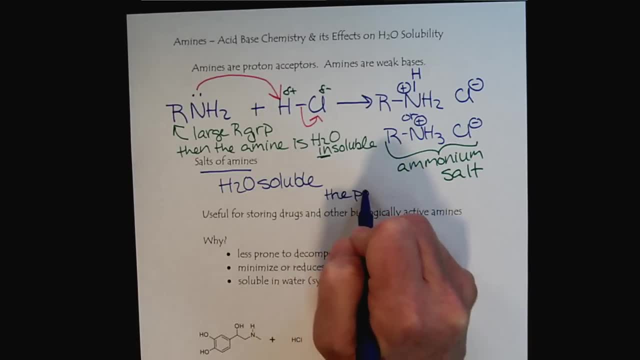 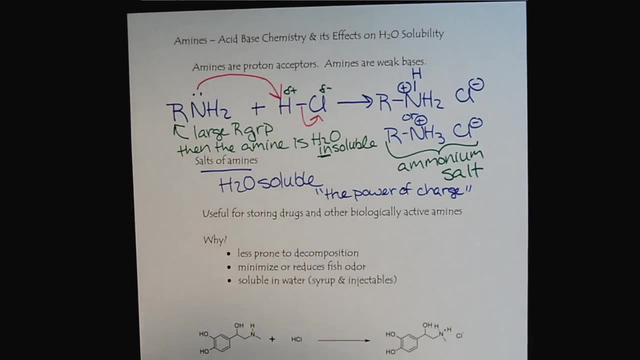 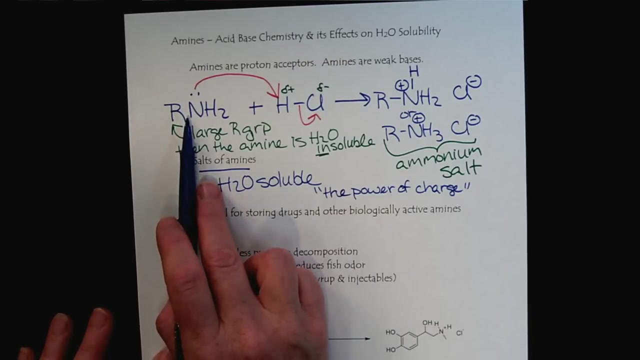 The power of charge. Okay, so for amines in particular, this is a very important thing, right? So we can go from an insoluble, a water-insoluble amine, to a water-soluble ammonium salt. 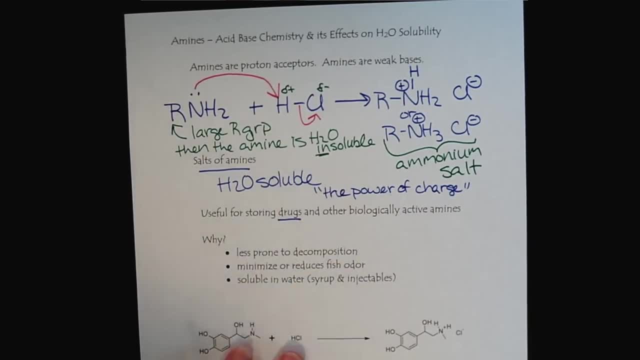 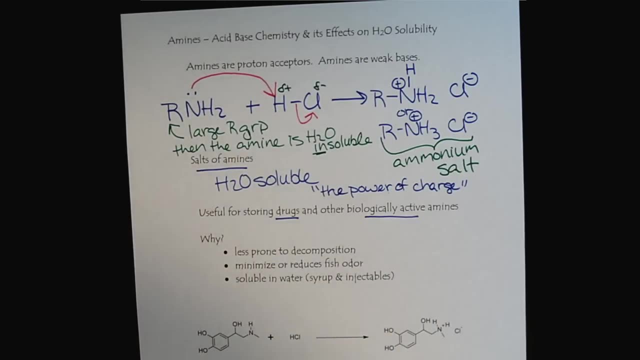 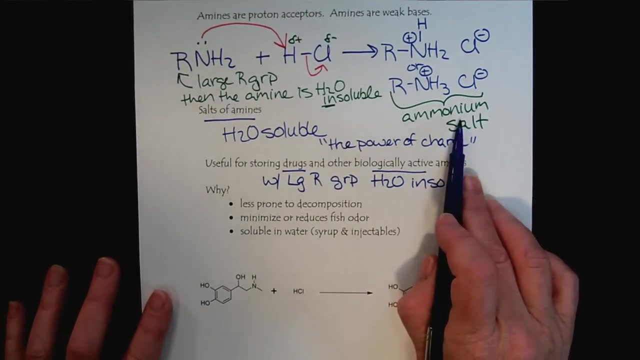 And many drugs are amines, and there's a ton of biologically active compounds that are amines, But they tend to have large R groups and so they're water-insoluble. Okay, so we want to make these amines into the ammonium salts. There are several reasons for this. The first one I've already mentioned: We want to create something that's water-soluble, so we can put it in a syrup to drink or inject it or put it in an IV. Another thing is that amines are very unstable and they're prone to decomposition. 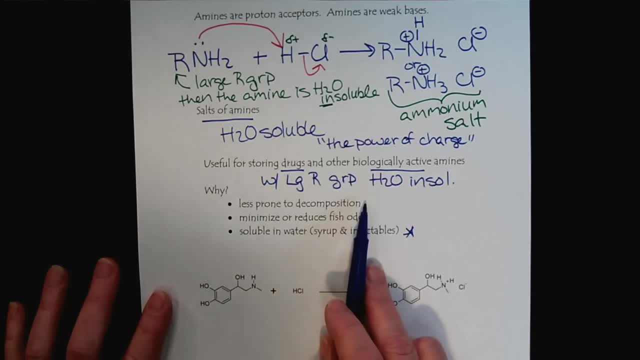 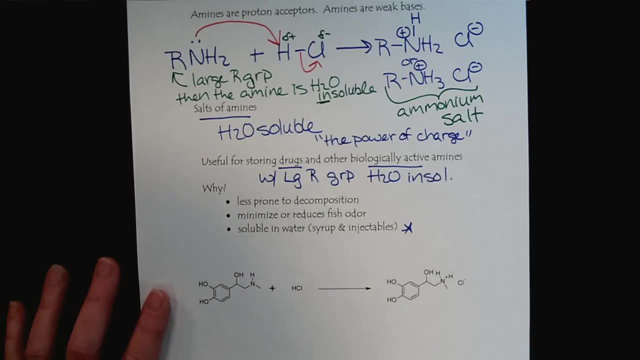 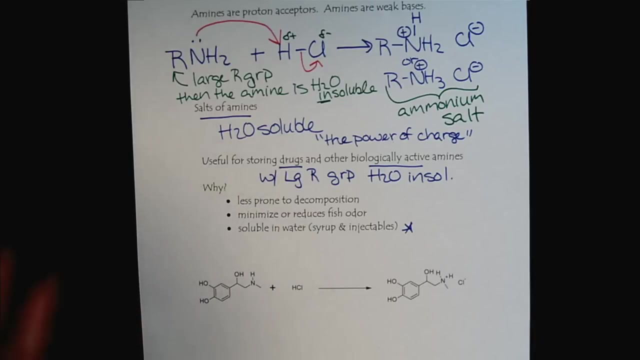 So the ammonium salts are much more stable. And, last but not least, amines tend to be very stinky and have like a rotten fish odor, And so when we make them into the salt, the odor goes away. So let's look at an example of how we can use the acid-base chemistry. 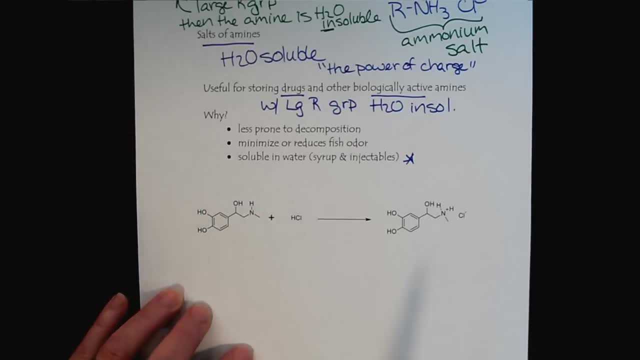 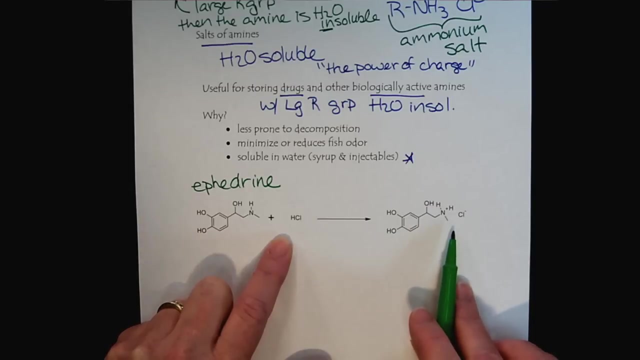 So let's look at a molecule of ephedrine, And then we're going to react it with hydrochloric acid, And so here is the ammonium salt, And so the name for the ammonium salt would be ephedrine hydrochloride. 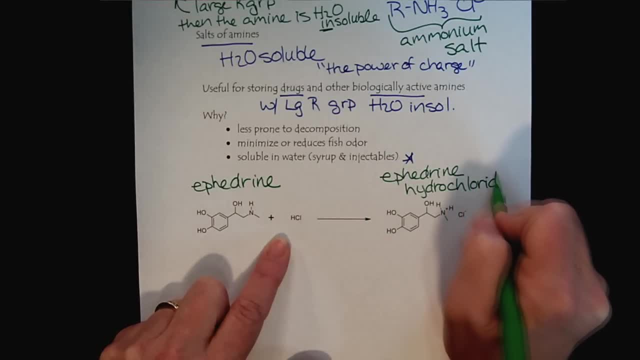 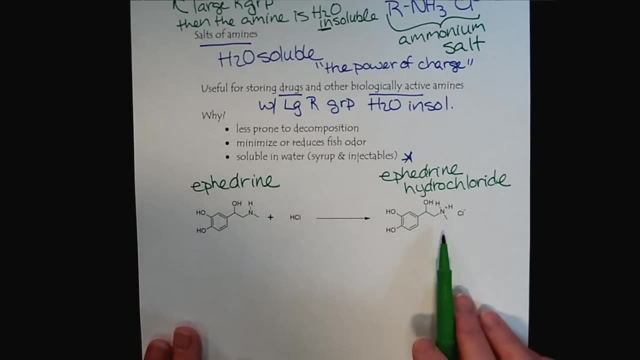 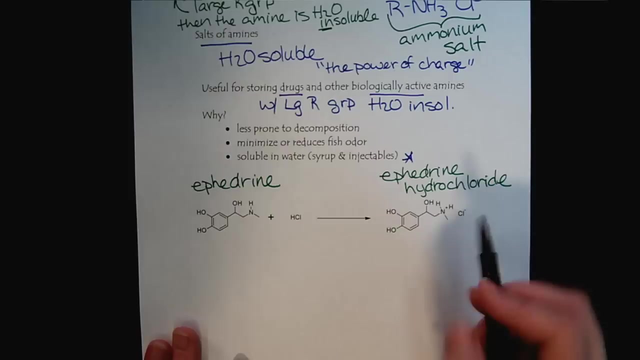 So we'll learn as we go on that a variety of acids could be used to create the ammonium salt, And so we let everybody know which acid we used. Now my software here is a little funky, so this bond got erased. 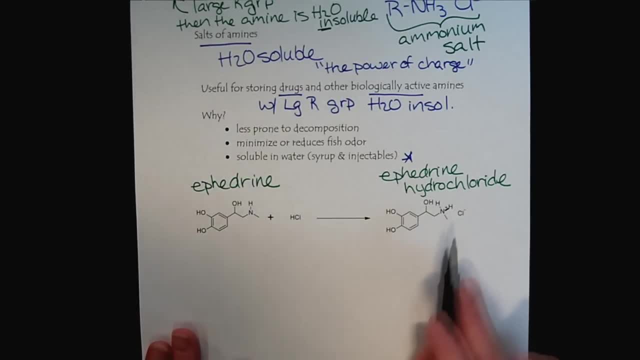 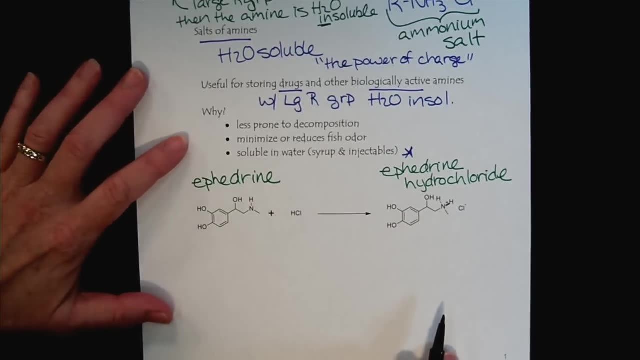 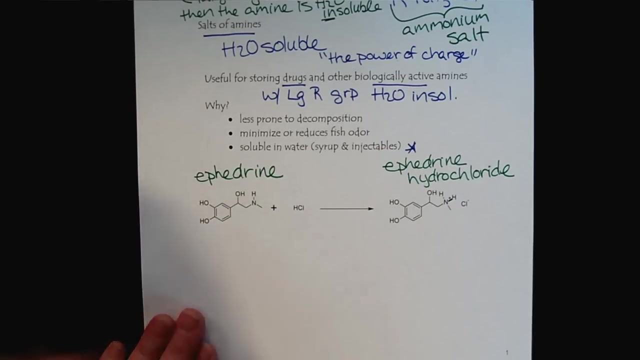 But nitrogen has the four bonds and that's why it has the positive charge, And this is our ammonium salt. So why is this chemistry so important? Well, let's look at the criteria. When we have ephedrine, and we would describe this as the, we would call this the free base. 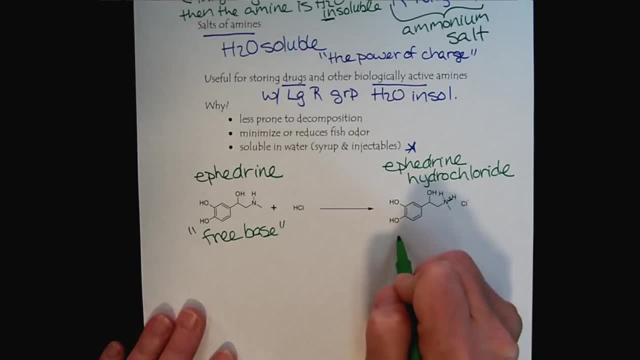 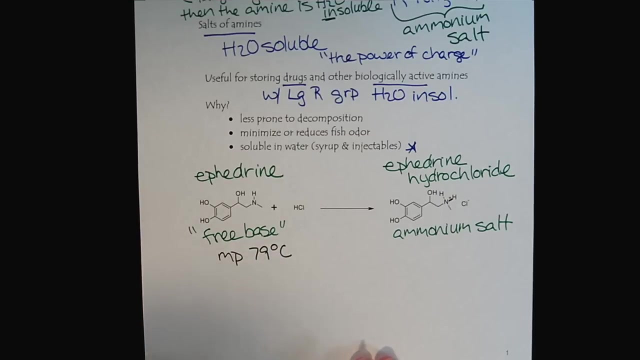 So the free base of ephedrine versus the ammonium salt, So the free base has a melting point of only 79 degrees C. So it's very fragile because this is a covalent, a molecular compound, Even though we have a lot of organic character here. it's still a salt, an ionic compound, and we know that ionic compounds have much higher melting points, So this helps to create more stability and less decomposition. The free base of ephedrine is very foul smelling. The common name of amines are like putrescine. 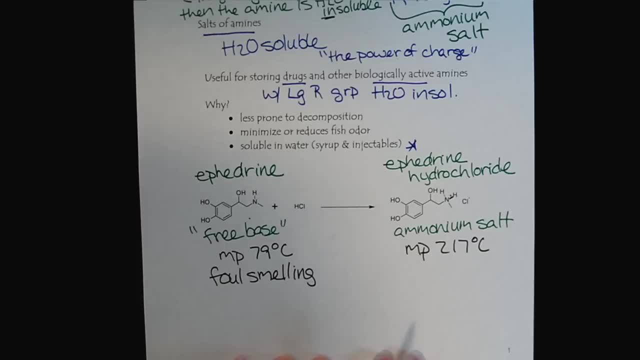 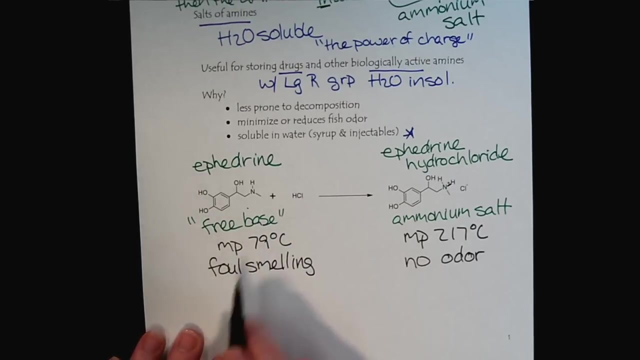 and cadabrine. If you've ever smelled rotting meat, you were smelling amines. The ammonium salt has no odor, Okay. So in addition to having a very low melting point, it's also chemically unstable versus the ammonium salt, which is very stable. 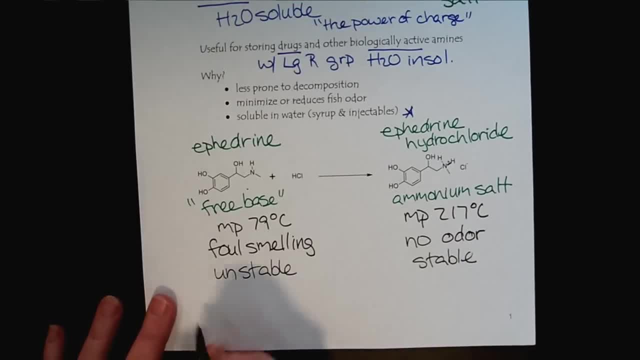 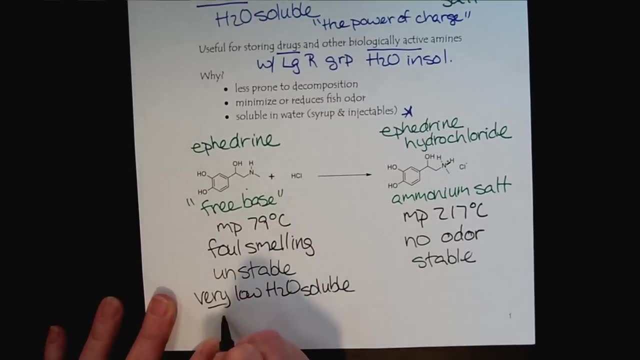 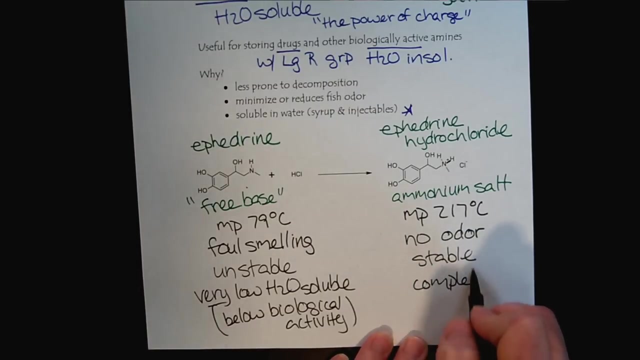 And, most importantly, that ephedrine has very low, very low water solubility- Right, Right below therapeutic help or below biological activity, Whereas the ammonium salt is completely soluble in water. So that's what helps us to be able to use these amines. 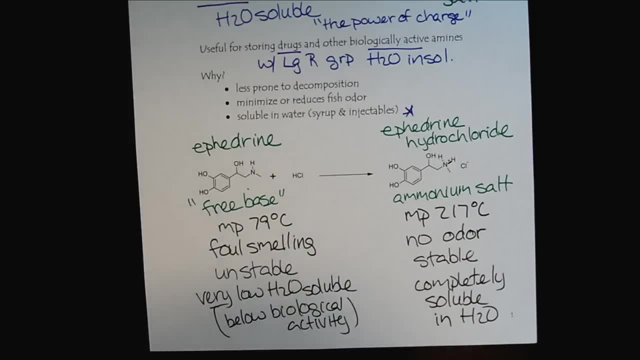 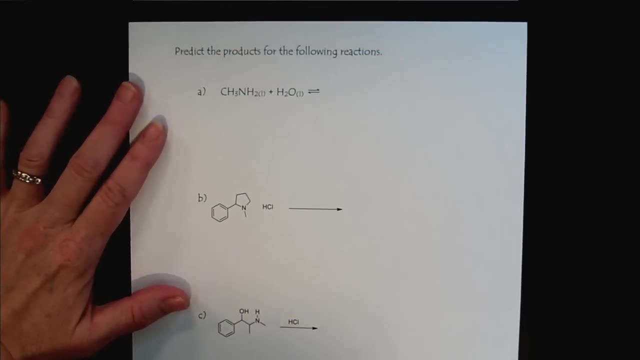 which are very biologically active in medicines. So now let's practice a bit more on this important acid-base chemistry. So we'll go to the next page, Alright, So in this first example we will just show amines with water. 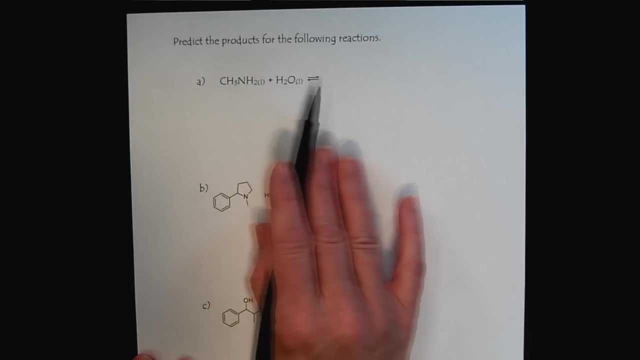 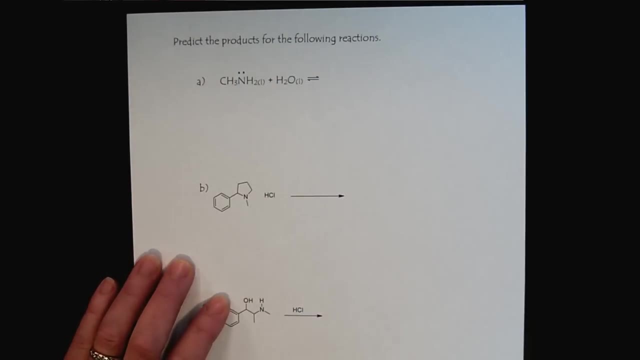 So here we have a weak base and a weak acid. So we'll use our equilibrium arrow And remember the bonding pattern of nitrogen, wanting three bonds and a lone pair, And I'll go ahead and draw the water molecule out, So remembering that it's this lone pair. 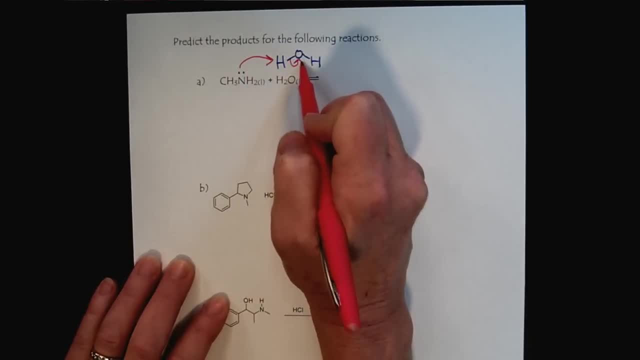 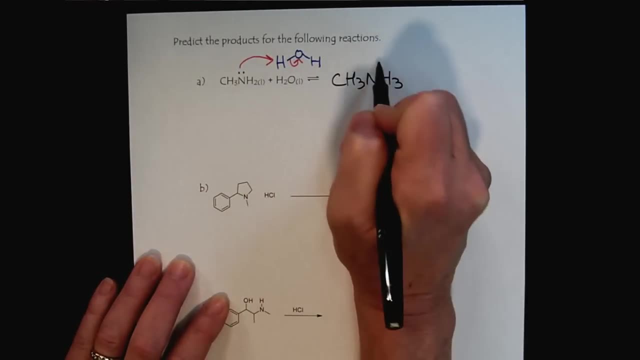 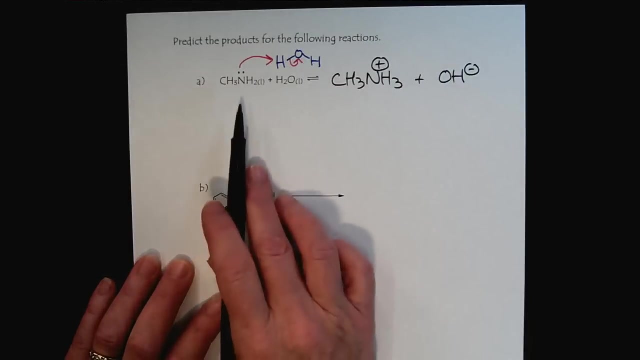 on the nitrogen, that creates its basic chemistry, And so we would end up with our methyl group, NH3 with a plus, And then here we would have hydroxide as the counter ion, And this can help us see why amines are weak bases. 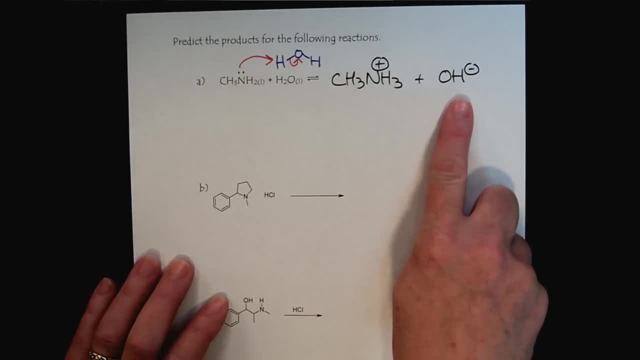 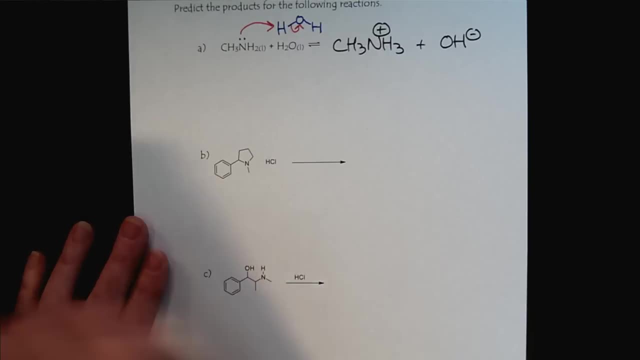 Because when we think about bases, we think about hydroxide. This next example: this is nicotine, And so there's our nitrogen. We will add the lone pairs And I think it's helpful to show the bond here And recognizing right. 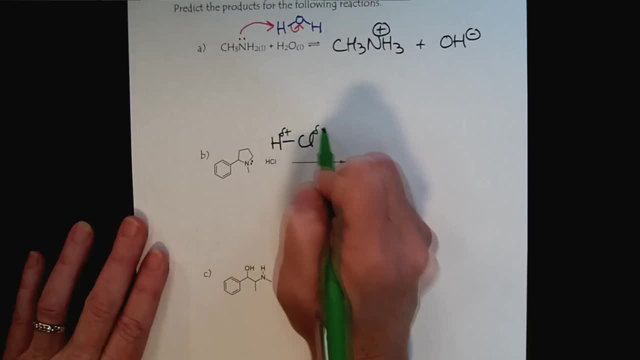 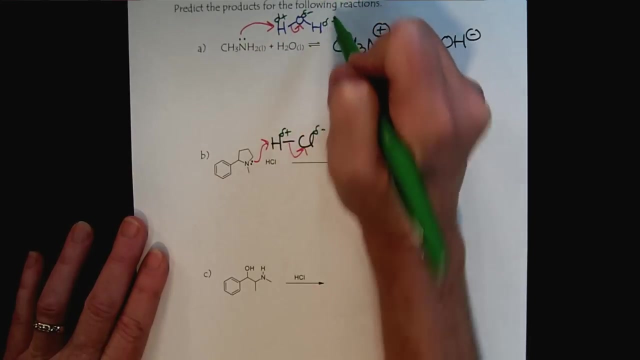 that we have once again. we have polar compound, And so those lone pairs on the nitrogen are attracted to the partial positive charge. I didn't show it on the water up here, But we'll just fill that in to be complete, Alrighty. 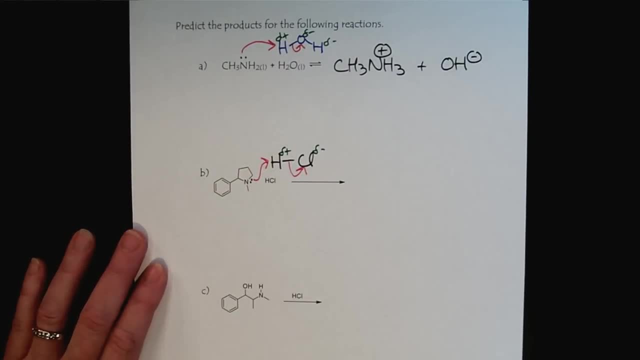 So various notice the similar pattern of reactivity And the R groups. you can see why. oh, it's really nice when we can just just put an R there and not have to draw all these carbons. But in this case, 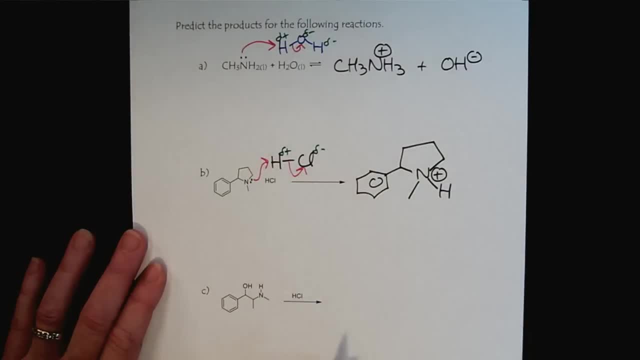 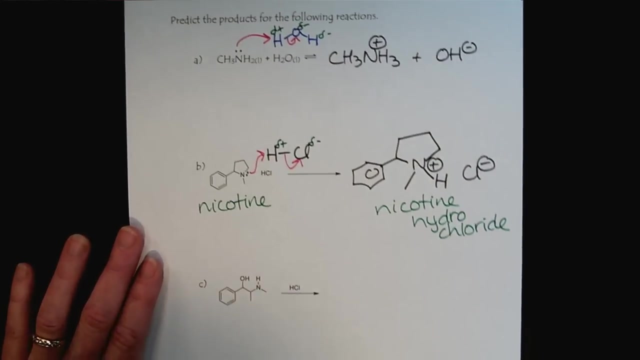 we'll show it. And so there we have. we have the ammonium salt. So here we definitely have our ammonium salt. So this is nicotine, And this would be described as nicotine hydrochloride. Alright, One last example to give you confidence when doing your homework. 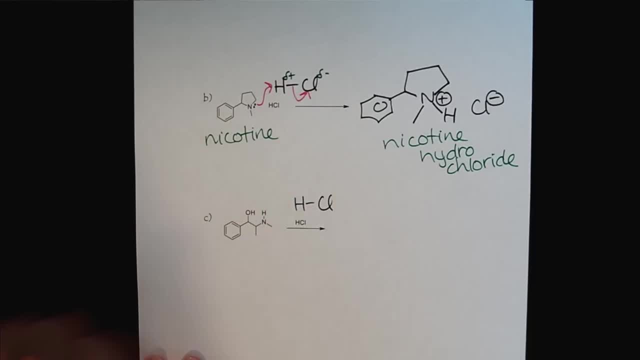 We'll go ahead and draw out HCl again And recognizing its polarity, And there's the lone pairs. Now remember that right. so alcohols are not acids or bases, So don't let that confuse us. We're focusing on amines. 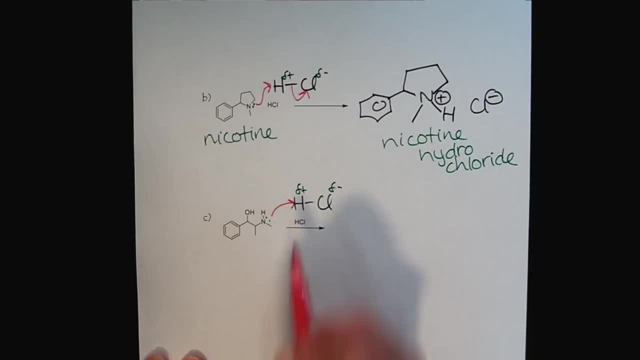 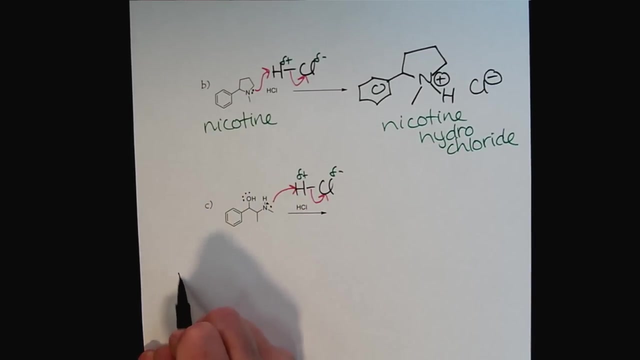 that lone pair on the nitrogen, Alright, So you can see that the hydrogen comes and reacts and forms a bond with hydrogen, Alright, If you're wondering, though maybe you're wondering like: but there's lone pairs on the oxygen, why don't they react? 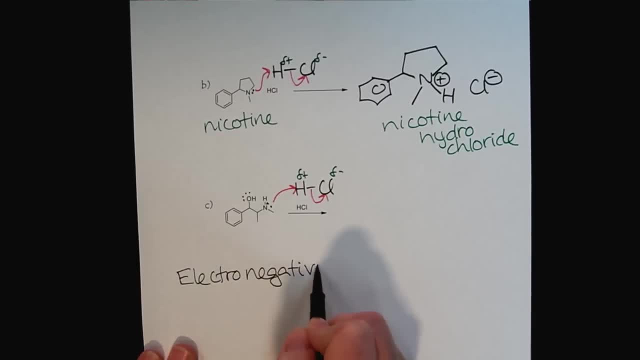 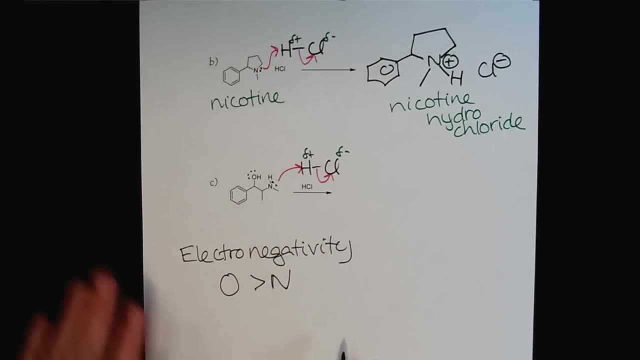 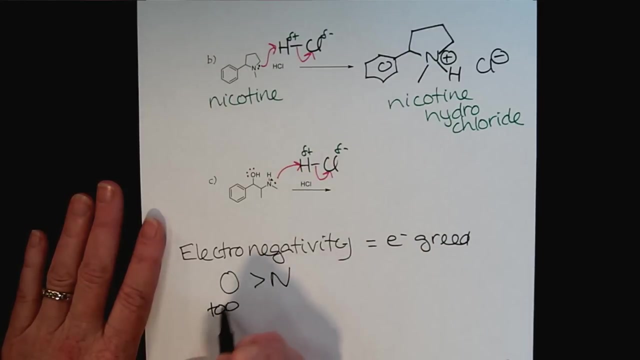 Let's remember our electronegativity. Who's more electronegative, right? Oxygen is more electronegative than nitrogen. Oxygen is more electronegative than nitrogen. Nitrogen is more electronegative than nitrogen Right. 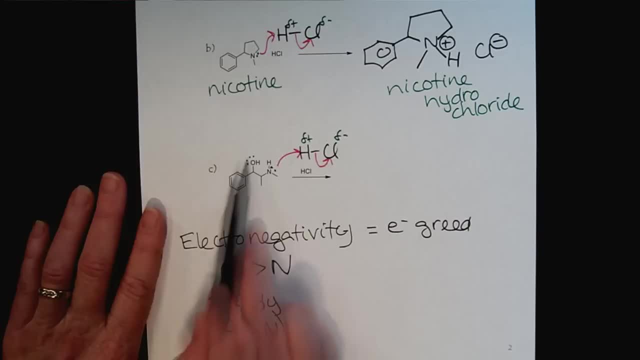 So that's an oxygen. So the lone pairs on the oxygen oxygen is not willing to share. But because nitrogen is less electronegative, these lone pairs have the freedom to go out and participate in an acid-base reaction. So now we'll draw our ammonium salt. 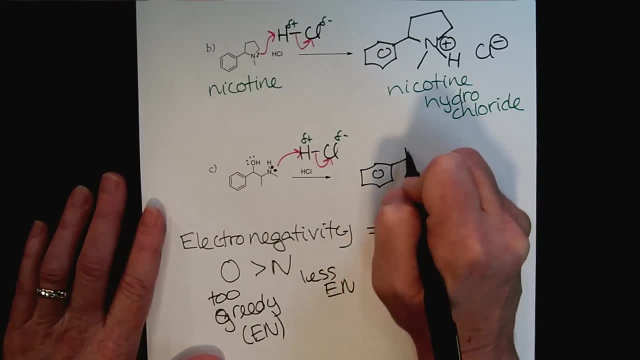 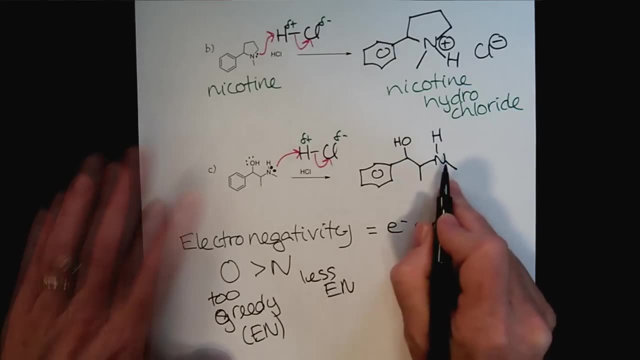 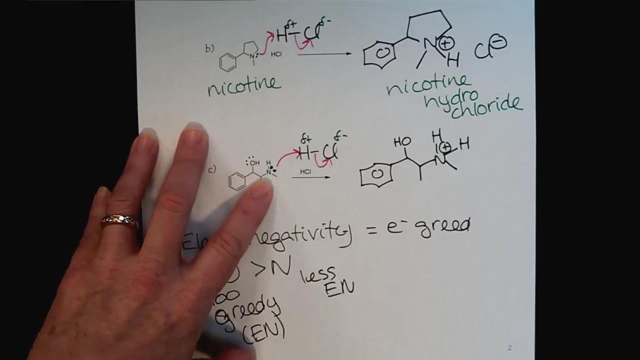 like we have. We'll draw our ammonium salt, like we have for the other examples, And so there was the original hydrogen, and now we would have the hydrogen that's connected through the reaction with the lone pair. And there we go. So once again,